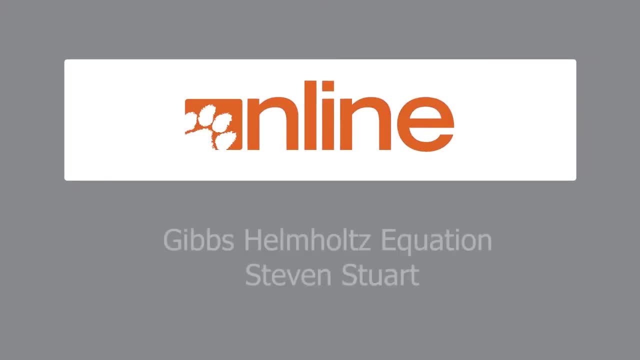 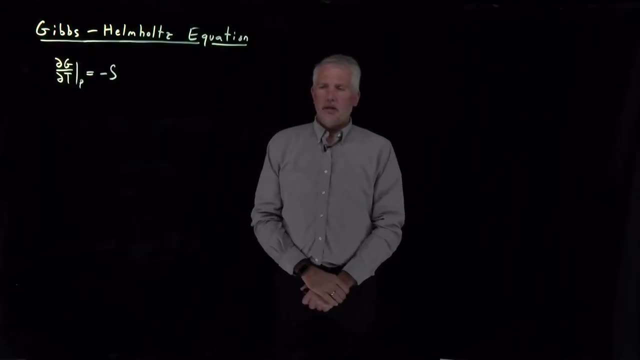 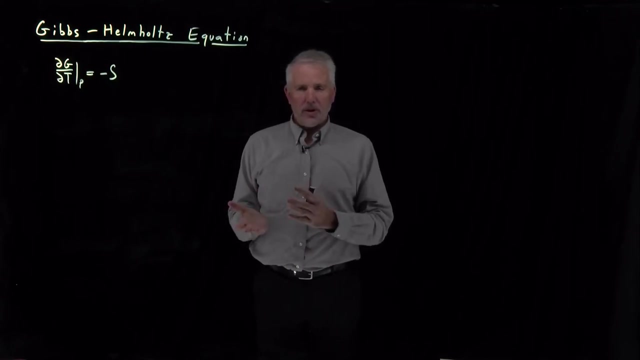 So we'd like to come up with a relationship between the Gibbs free energy and the temperature So we know how much the Gibbs free energy is going to change when the temperature changes. We have such a relationship but that Gibbs free energy changing with the temperature. 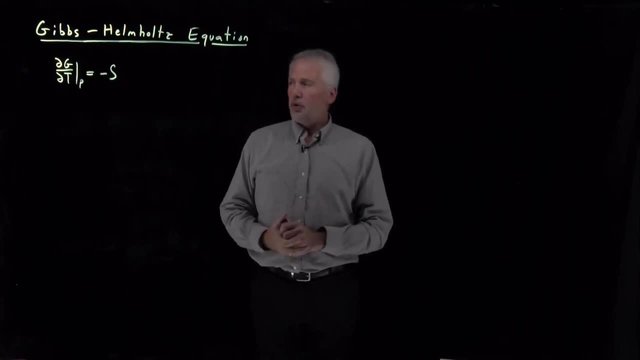 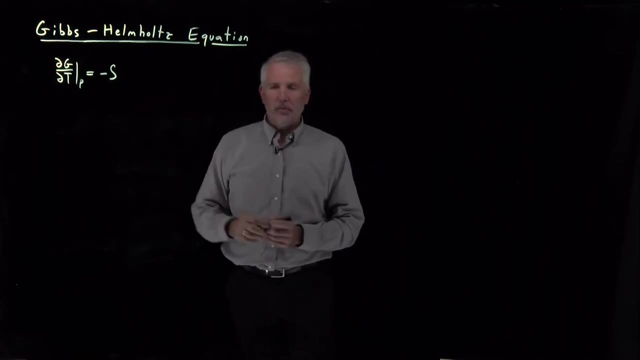 proportionally to the negative of the entropy. that's a true thermodynamic relationship, but it's not the most convenient one. So we'd like to come up with a more convenient relationship between the Gibbs energy and the temperature, and that's going to be this Gibbs-Helmholtz equation. 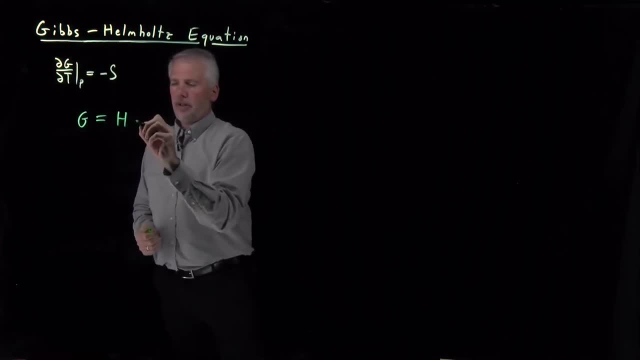 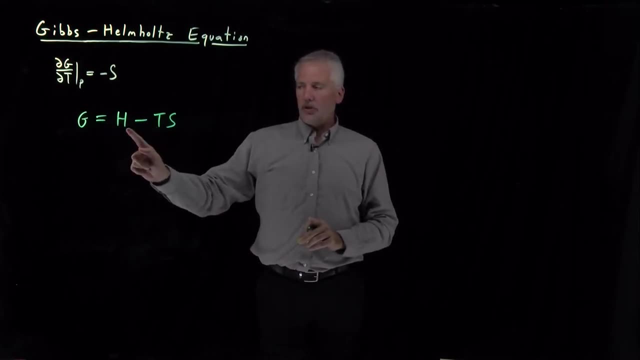 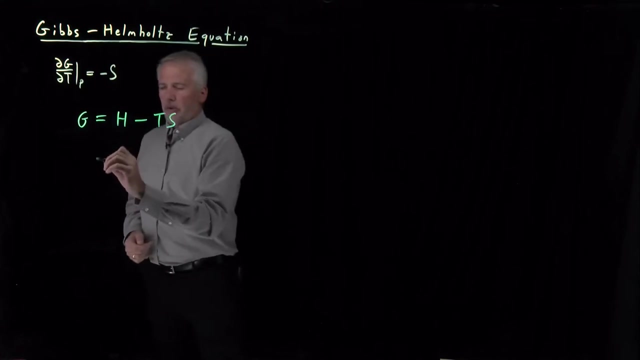 So we can start with our definition of the Gibbs free energy. That's certainly one thing that tells us how the Gibbs energy is related to the temperature, although there's also a temperature dependence hiding inside this enthalpy and hiding inside the entropy. What I'll do next is I'll go through and divide on the left and right side of this. 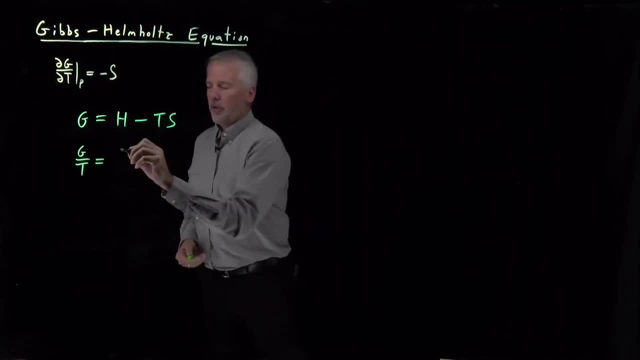 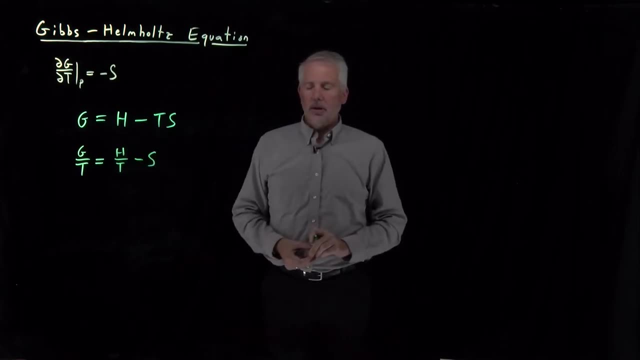 equation by temperature. So G divided by T is going to be equal to the enthalpy divided by T minus the entropy. or I've divided away this temperature. So that's a relationship between- not the Gibbs, free energy and enthalpy and entropy. but 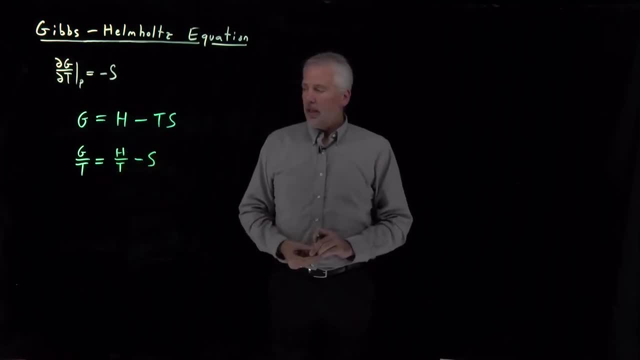 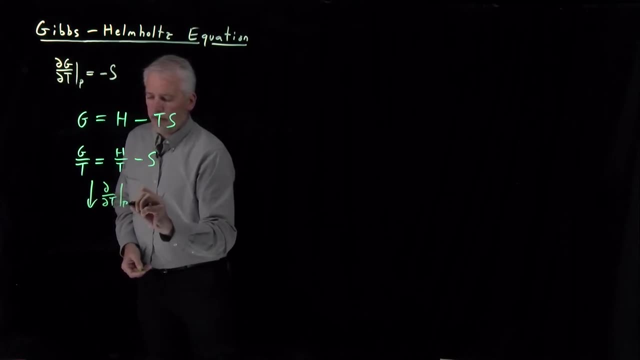 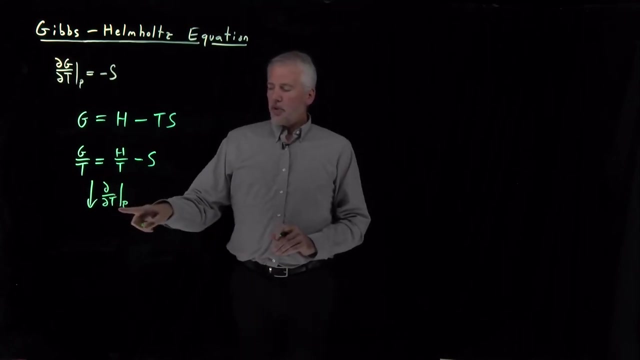 G over T and how that depends on the enthalpy and the entropy. So this expression: now, if I take the temperature derivative of each side of this expression turns out, we'll get something very useful. So take the temperature derivative at constant pressure. 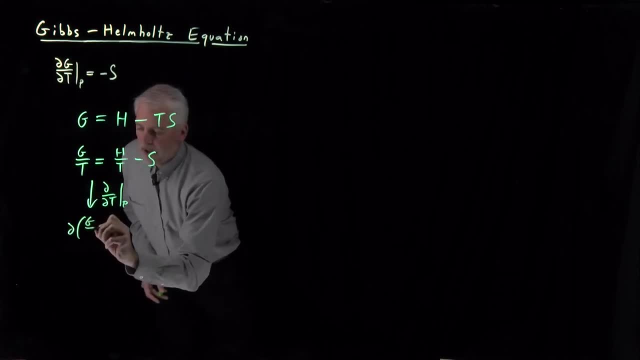 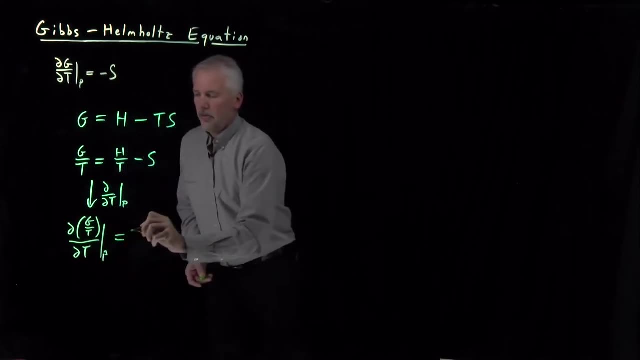 When I do that on the left, I'm just going to write the derivative of G over T with respect to T, at constant pressure On the right. I'll do that slightly differently. I'm going to do that on the left. I'm going to do that on the right. 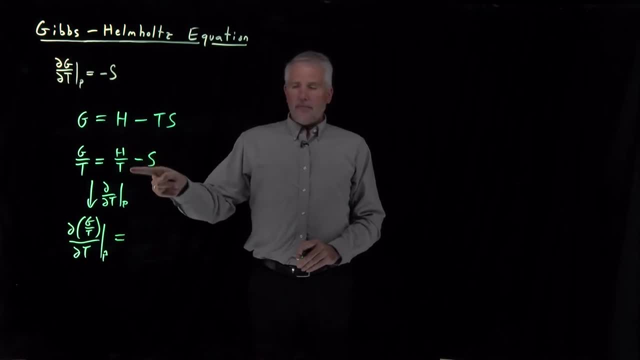 I'm going to do that on the left, I'm going to do that on the right, I'm going to do that on the left. So if I do that slightly differently, the derivative of this ratio H over T, I can use the product rule and say the temperature derivative is first. taking the derivative. 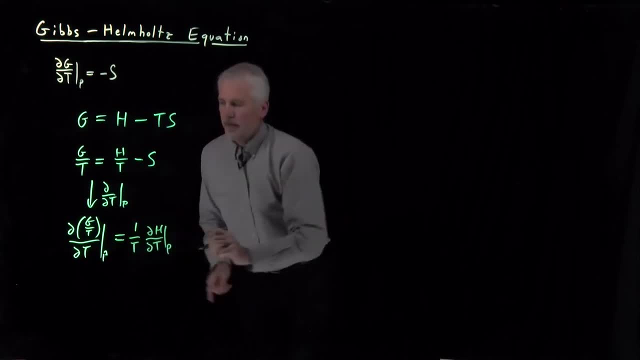 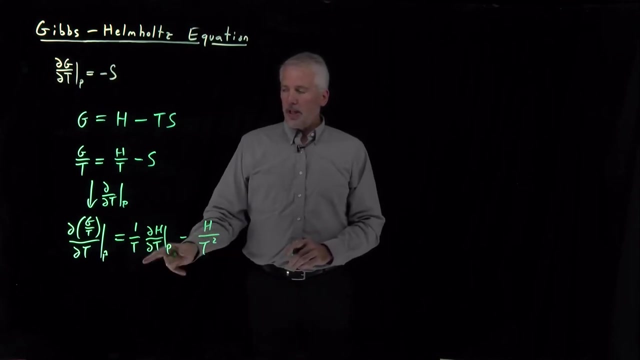 of the numerator, It's 1 over T times the derivative of H. and then product rule says also take H and then the derivative of the 1 over T is negative, 1 over T squared. So these two terms together are the temperature derivative of H over T. I've got the temperature. 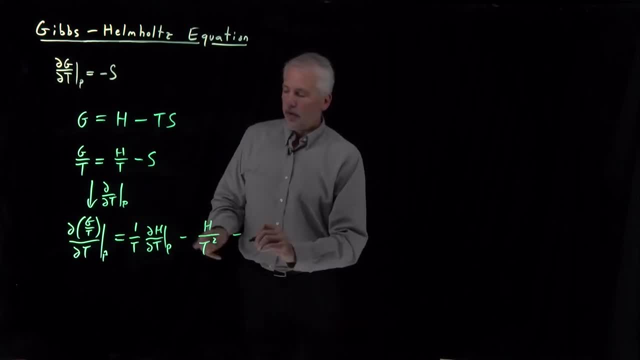 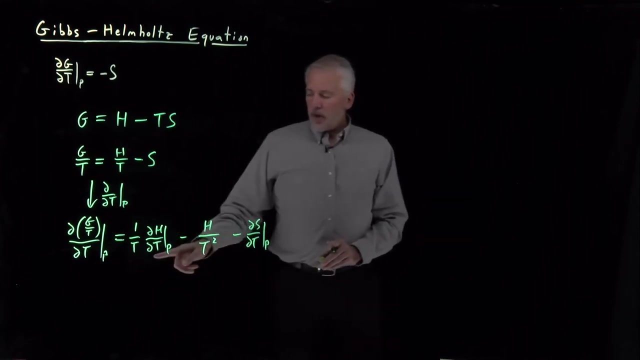 left this negative S, So the derivative of S. I'll go ahead and write dS, dt at constant P as our derivative of S with respect to T at constant pressure. So I've evaluated the derivative on the right-hand side, except we actually know what two of these 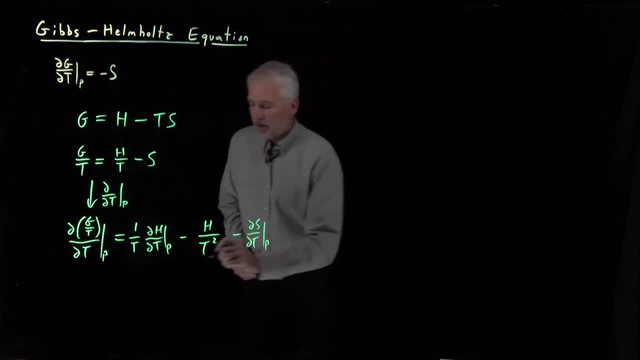 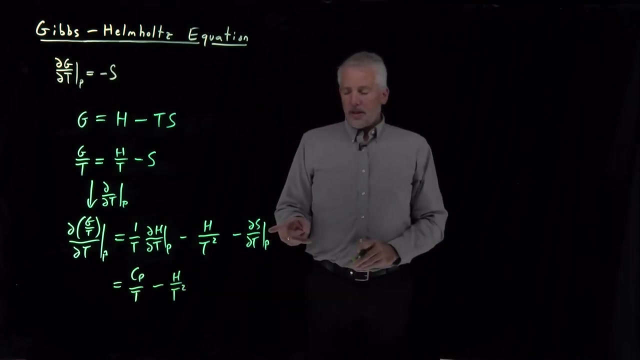 derivatives are: dH, dt at constant P should look familiar. That's by definition. that's the heat capacity at constant pressure. The second term: we can't do too much with minus H over T squared. The third term: we also know something about this: dS, dt at constant P. that's the derivative. 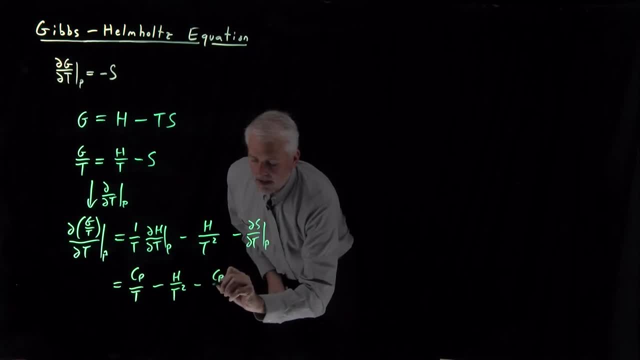 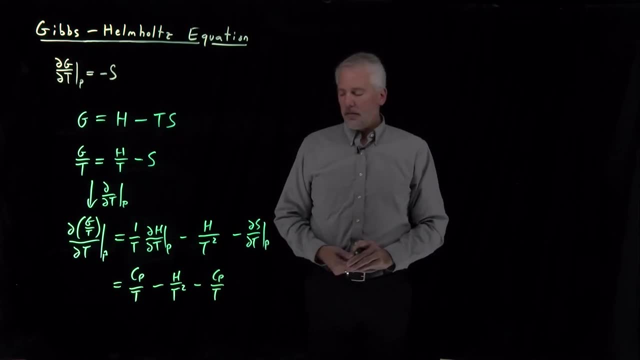 we've seen before. That is in fact heat capacity divided by temperature. If the derivative's at constant pressure, it's Cp, the constant pressure, heat capacity divided by temperature. So notice now that the Cp over T in the first term and the negative Cp over T in the second. 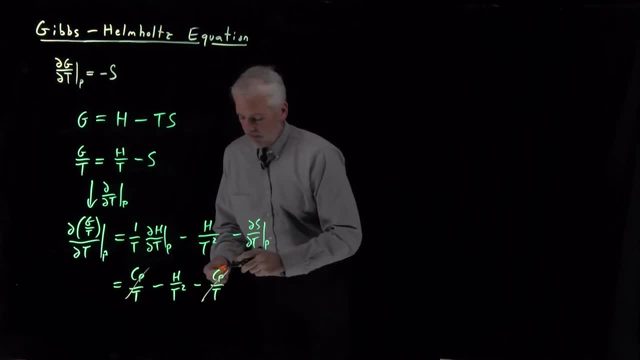 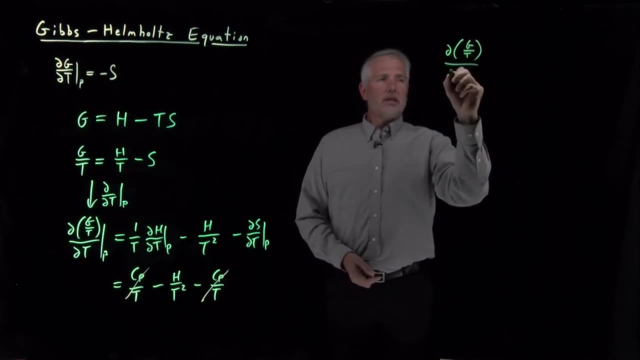 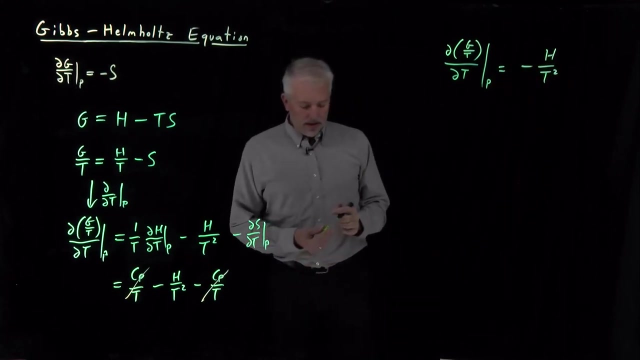 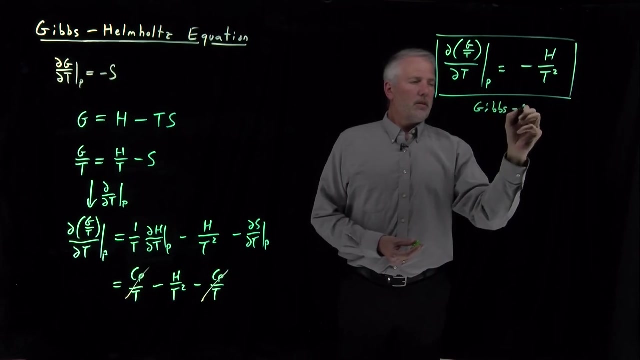 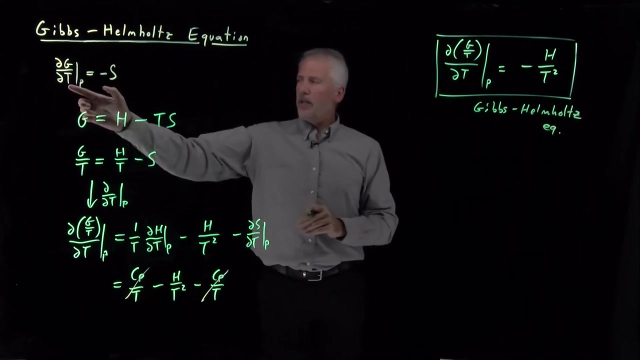 term. those cancel each other And what we're left with- I'll go ahead and write up here- is this result, which is called the Gibbs-Helmholtz equation. It's a true statement, but not terribly convenient, That the free energy 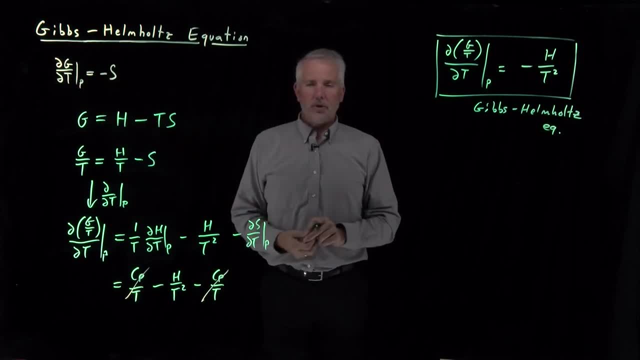 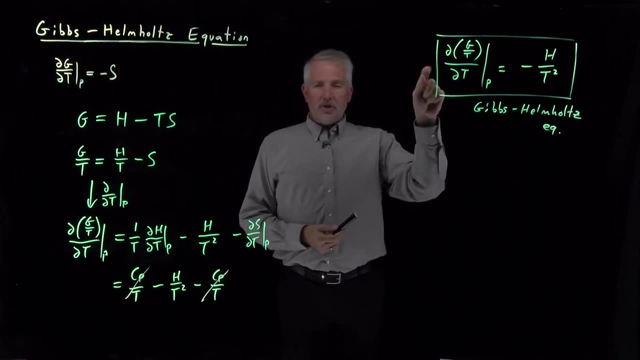 The free energy changes with the temperature proportionally to the negative of the entropy. It's also a true statement, more convenient to use that if we're not interested in G, if what we think about is G over T, this quantity Gibbs free energy divided by the temperature. 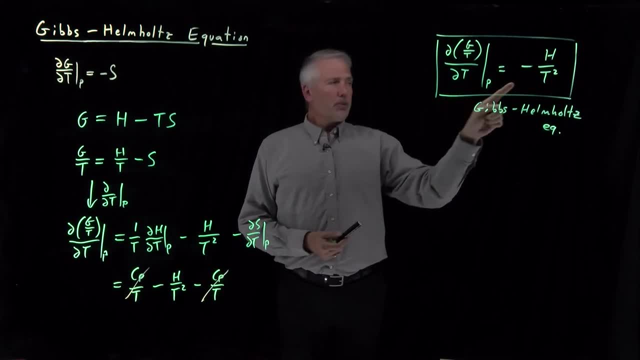 that quantity changes as I change the temperature proportionally to minus H over T squared. That looks like a more complicated relationship but it's easier to use in practice because it's fairly simple to go into a lab and determine the enthalpy of the energy.